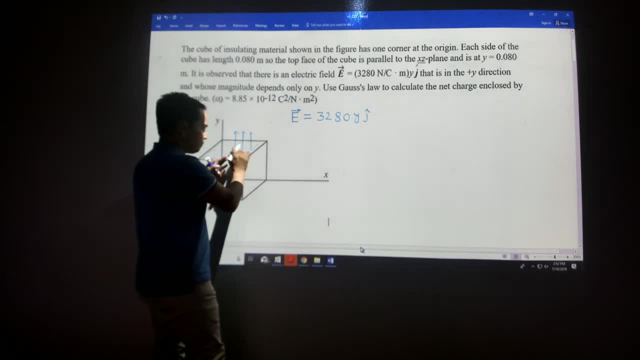 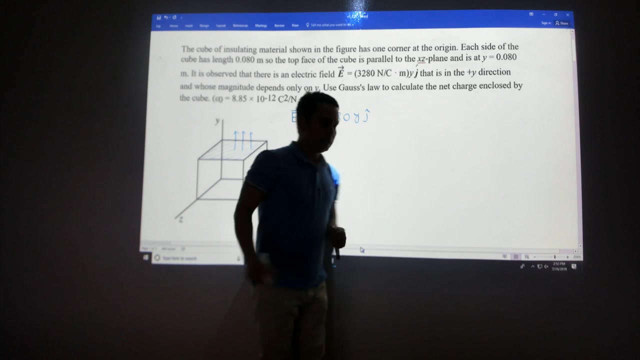 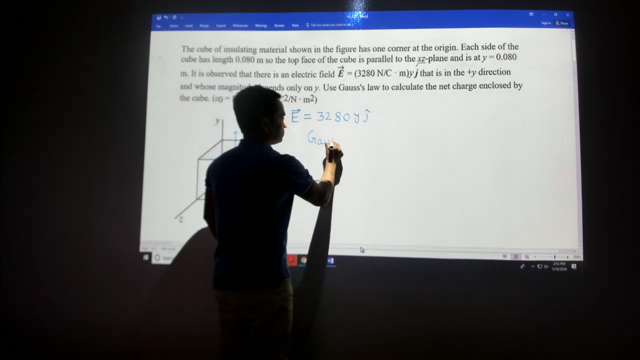 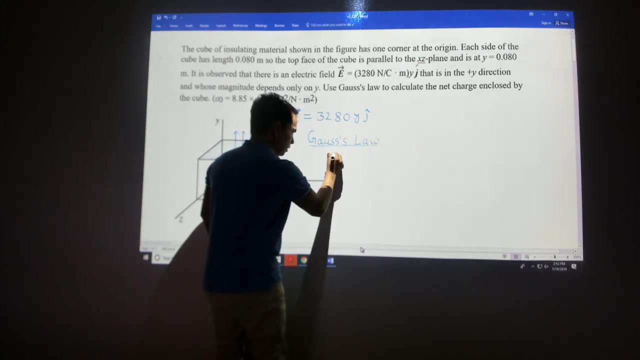 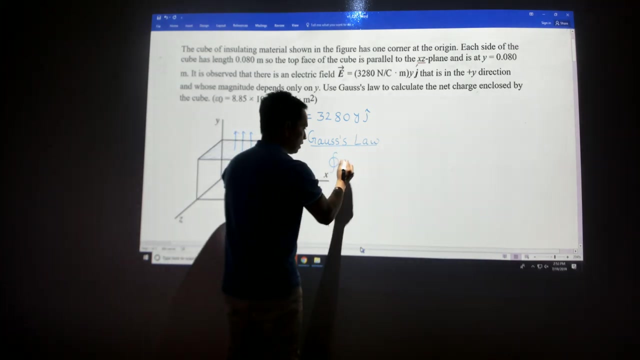 So all the electric flux is only passing through this face here, Through the top face. So how do you use the Gauss law to calculate the charge enclosed within this cube? What does the Gauss law tell you? This law tells you the total charge enclosed within a closed surface, the total flux. 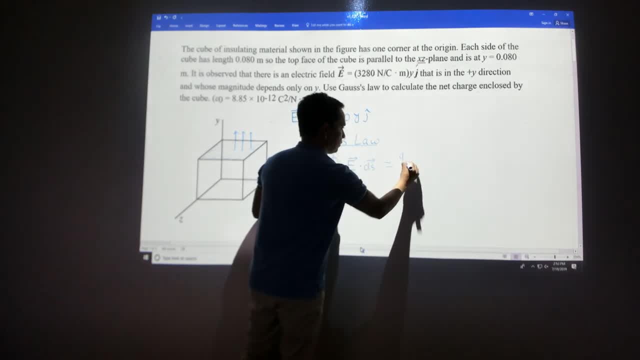 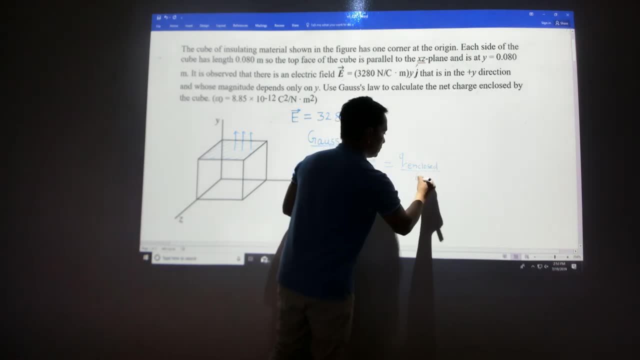 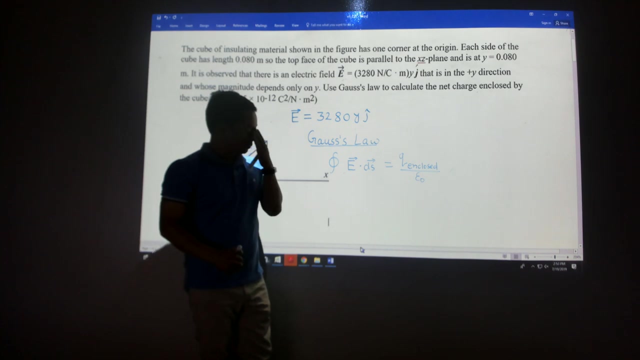 is given by Q, enclosed, divided by epsilon naught. We know this is a constant quantity, Alright, So what do we need to know now? So we have to find this integral here. But the life is so easy here if you just pay attention. 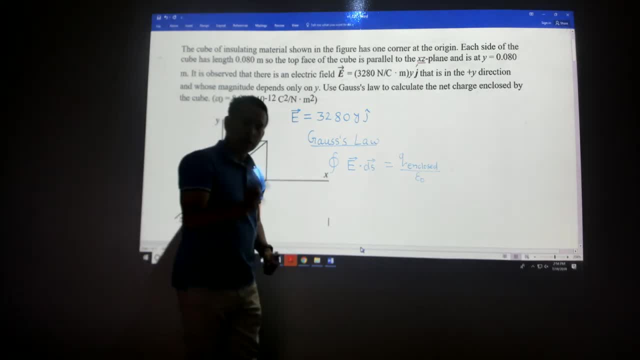 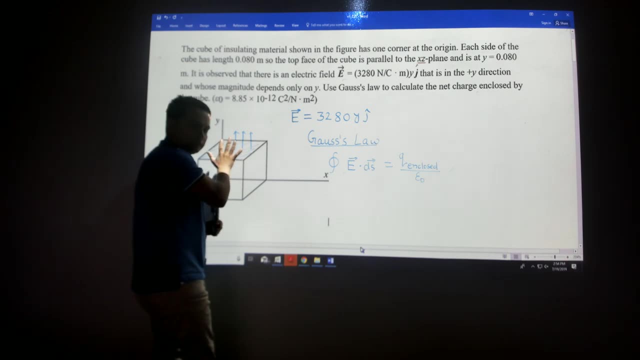 So this is the electric field and, if you look, this one is the elementary area. So, as I mentioned, the electric field only passes through the top face. There is no electric field coming out of this surface or this surface, or through this surface or to the back surface. 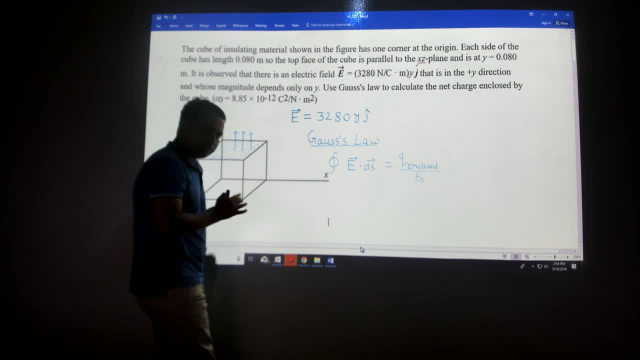 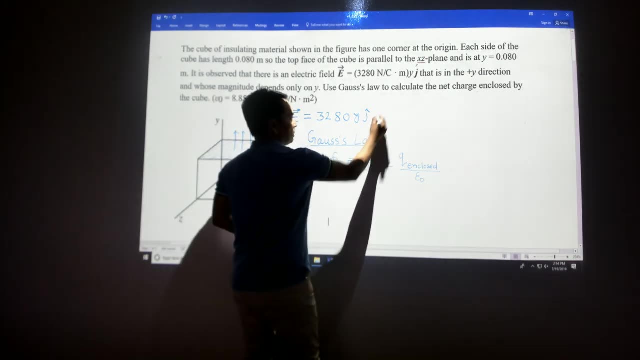 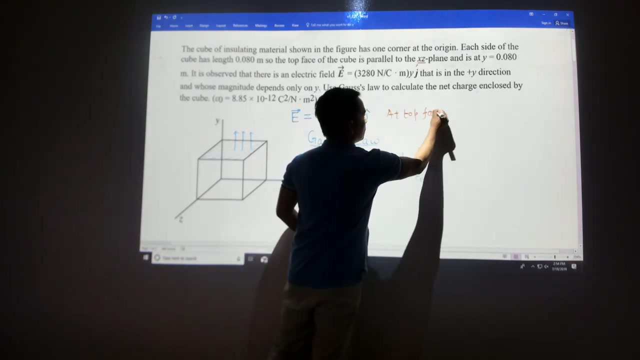 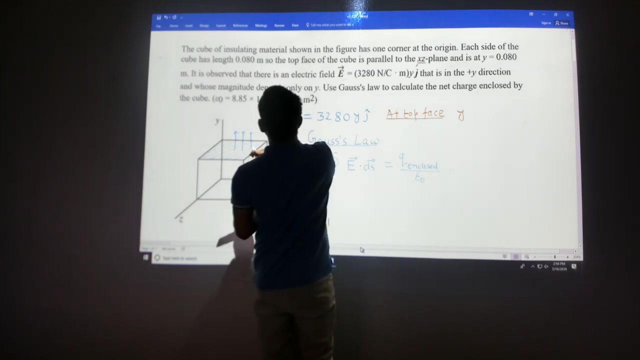 So let's find out what is the electric field value at this top, the top side. I can write it down here: At top face y is the value. the length or the height is given. Each side has 0.080.. 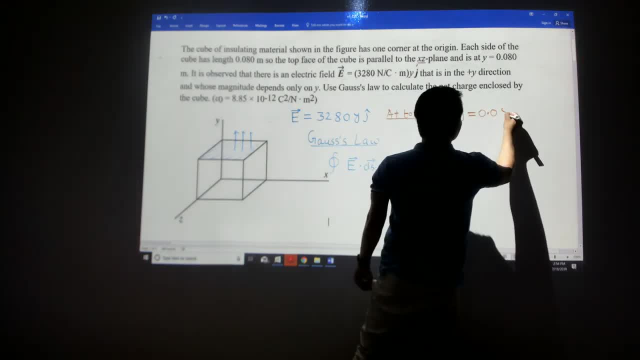 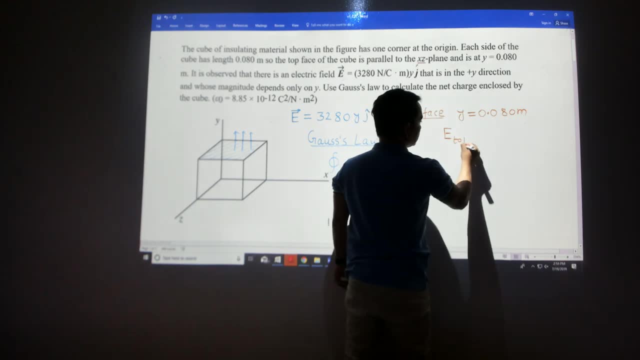 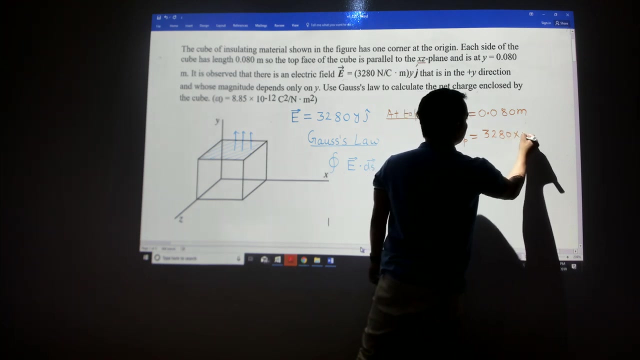 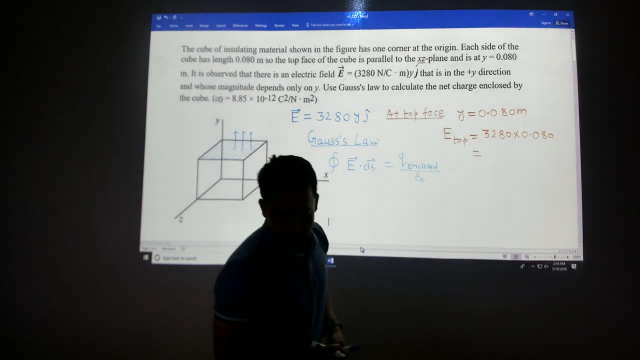 0.080 meter. So the electric field value at the top- I'm just writing it down here- is given by 3280 times 0.08.. So just have to calculate this number here. The number you will get is: 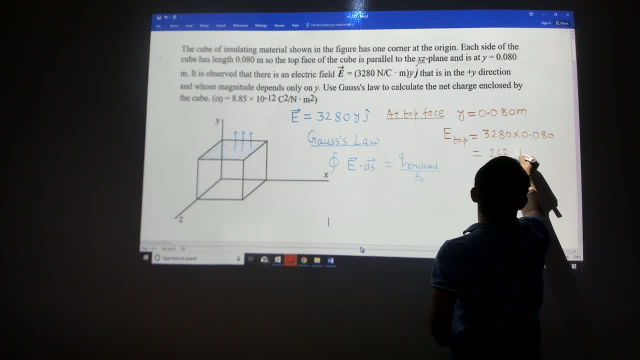 262.4 Newton per Coulomb. That's the number you get, Which means this value. this is the electric field value, this top surface. here We now have the electric field value. Now how do we calculate the total flux? 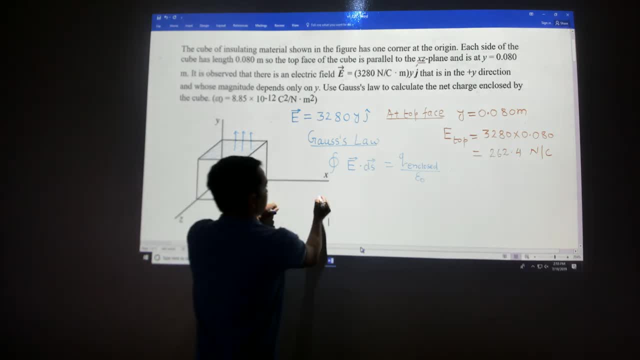 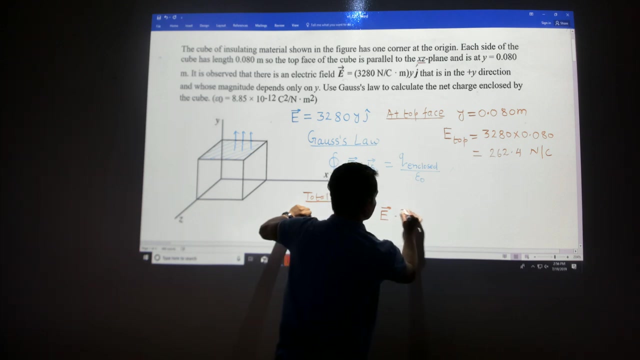 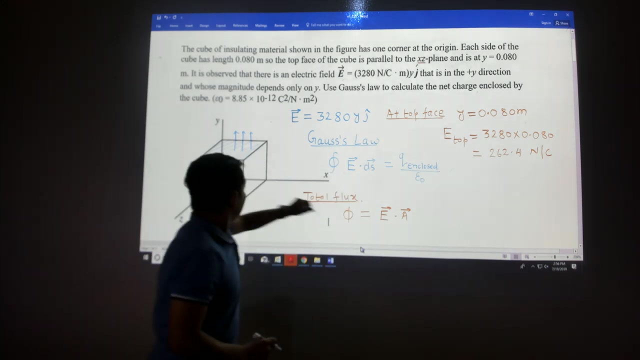 The total flux is passing only through this area. So the total flux- the total flux- we denote this total flux by 5, is the electric field at that point times the area, This area. Okay, This is exactly the same thing here. 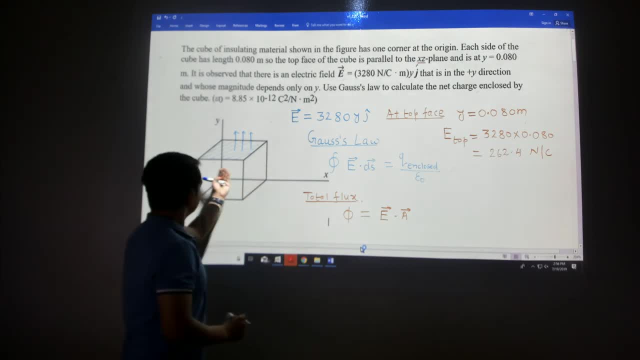 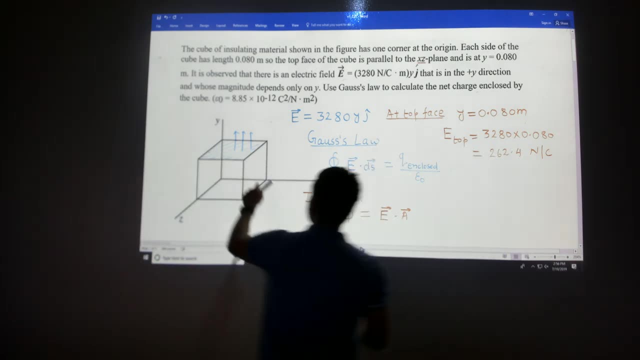 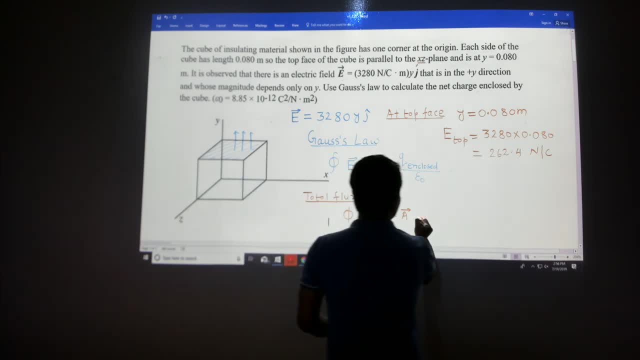 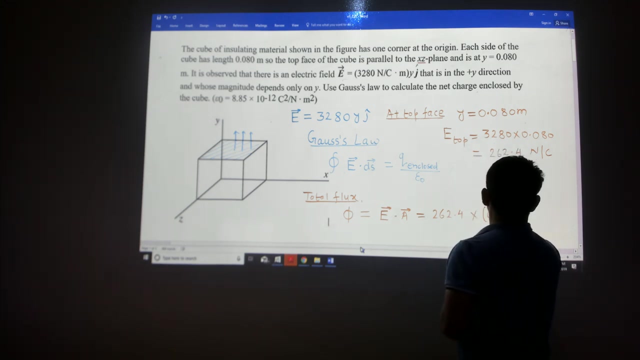 These two are parallel. So the electric field value at this point is 262.4 times. what is the area? at this point, The area is 0.080.. 0.080.. 0.080 times 0.080.. 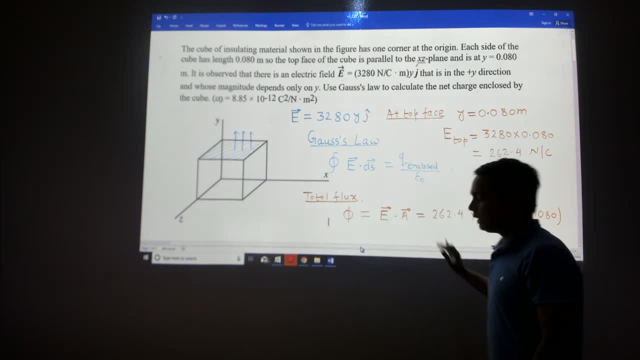 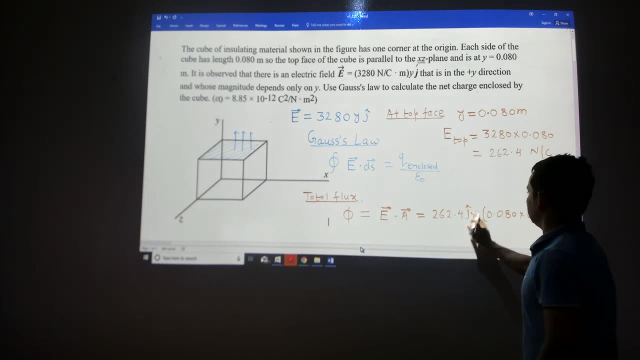 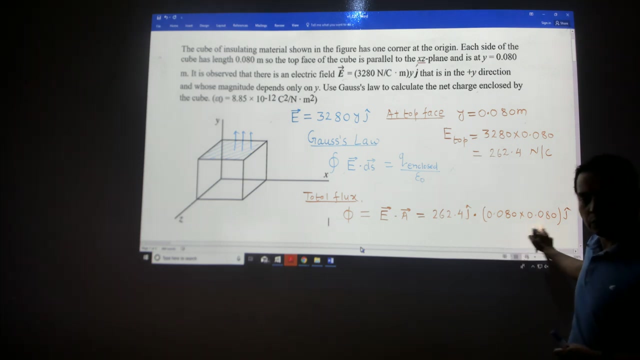 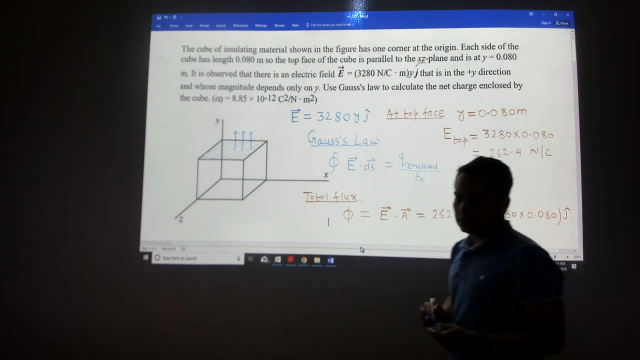 Remember, just to be more specific, what I'm going to write down here: a J vector times here, Just to be more specific, Because both are oriented along the Y direction. That's why I'm taking J vector and J vector. Let's now. 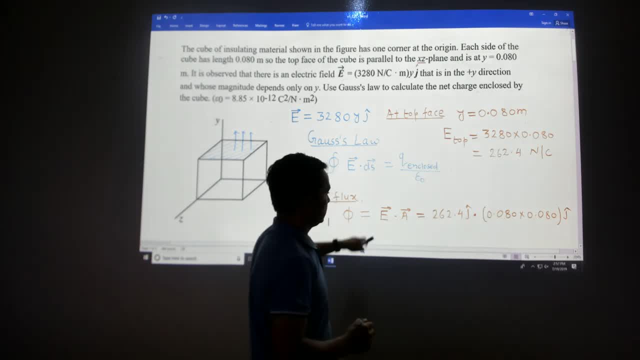 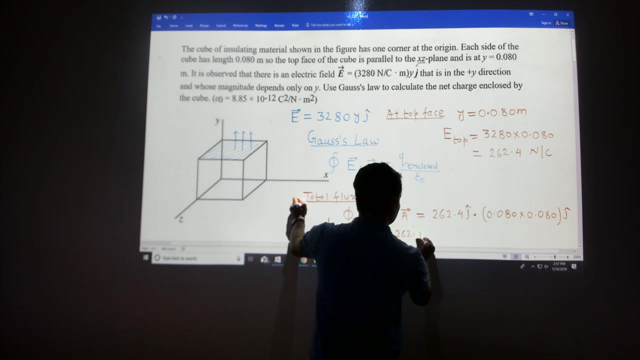 and this is the total flux. Let's calculate this number now. So this flux has to be equal to charge enclosed, divided by epsilon naught, And whatever the number, you get, 262.4 times 0.080.. 262.4 times 0.080..